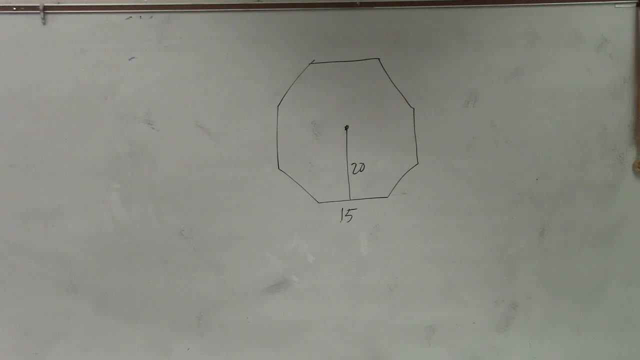 Okay, so in this example, what I will do is read your text message out loud. Now we went over the formula, I believe, and the formula one thing we noticed talked about this is: this is a regular octagon, And what we're talking about a regular octagon is the fact that all the sides are equal. 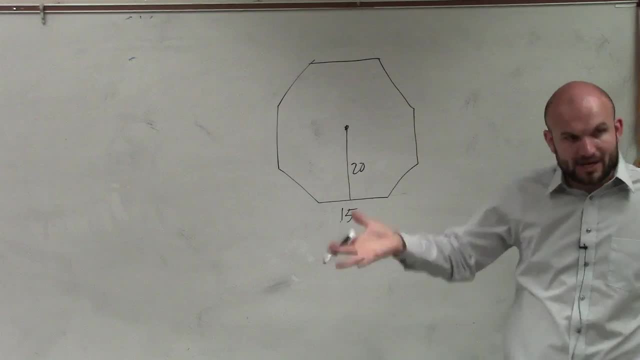 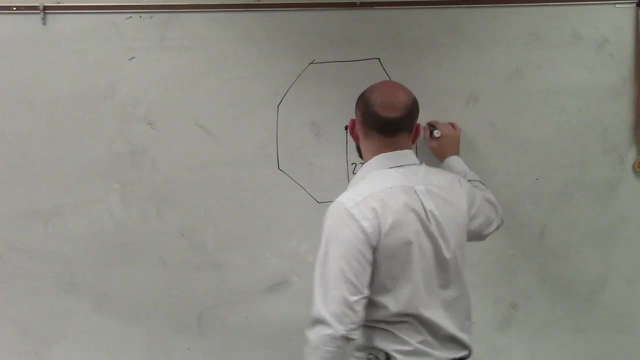 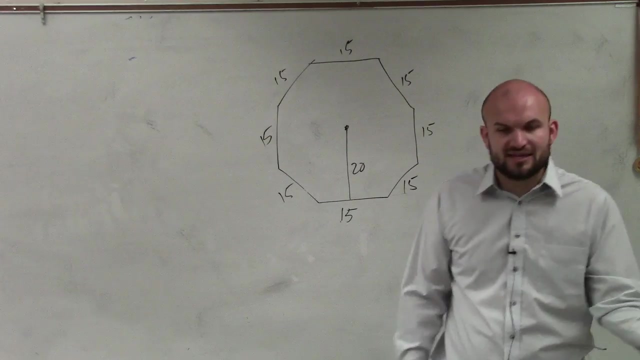 measure as well as all the interior angles. That's what makes a regular polygon, And in this case it's an octagon, because it has eight sides. So if the length of this is 15, all of these sides are 15.. Would everybody agree with me on that? Okay, now we talked about how to find the area. 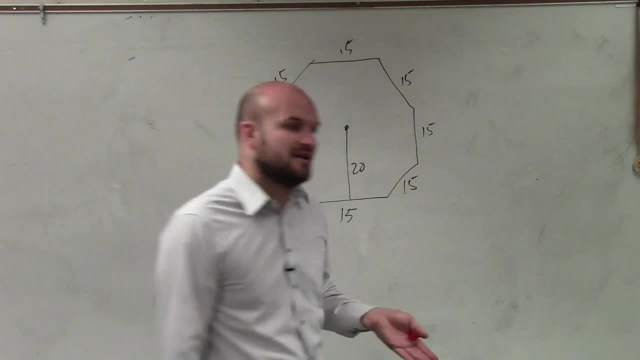 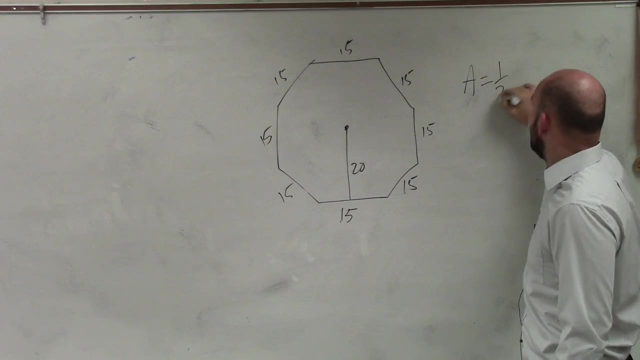 of a parallelogram, we talked about how to find the area of a triangle, and we talked about how to find the area of a circle and a trapezoid. So the area for any regular pentagon equals one half a times p. all right, Well, remember, a equals the apothem. 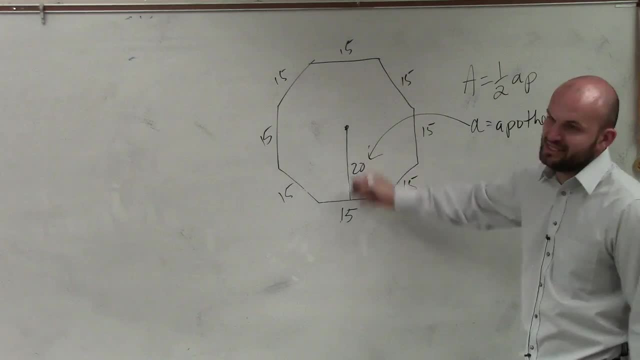 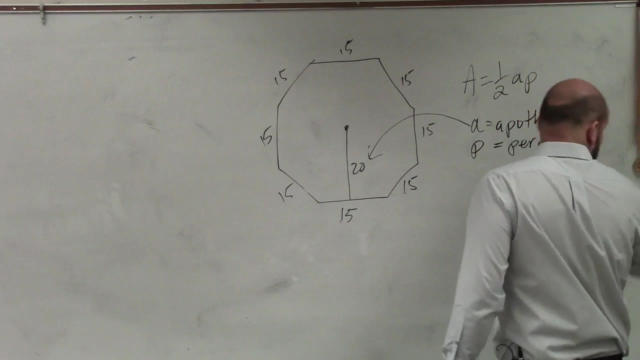 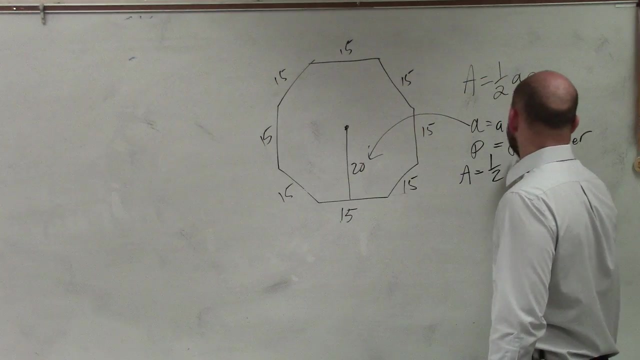 And the apothem is the distance from the base to the center of a regular polygon, And p equals the perimeter, all right, So therefore you guys can see that the area equals one half 20 times. now. I need to figure out the perimeter Now. I could add 15 up all the time. 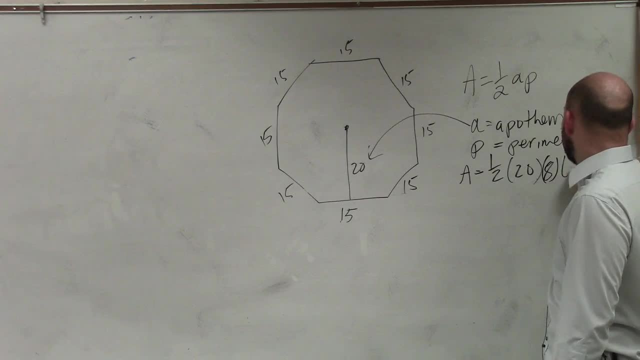 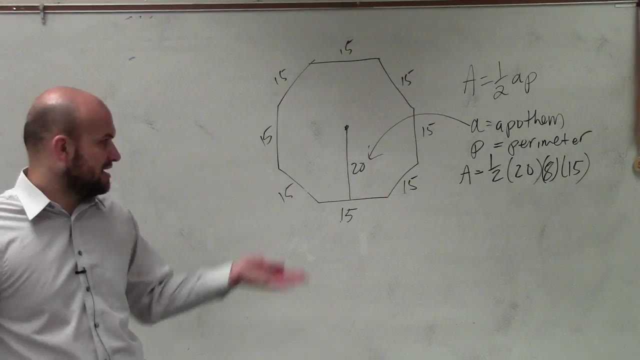 or you could just say 8 times 15, right? Is adding 15 eight times the same thing as adding 15 up all the time? No, it's not the same thing. It's the same thing. It's saying 8 times 15, right? So that's going to end up being 120.. 8 times 15 is 120. Times one. 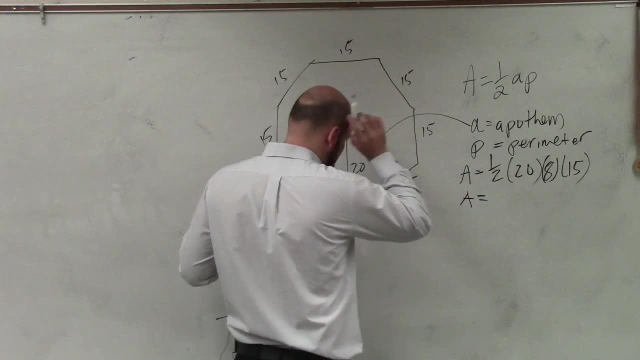 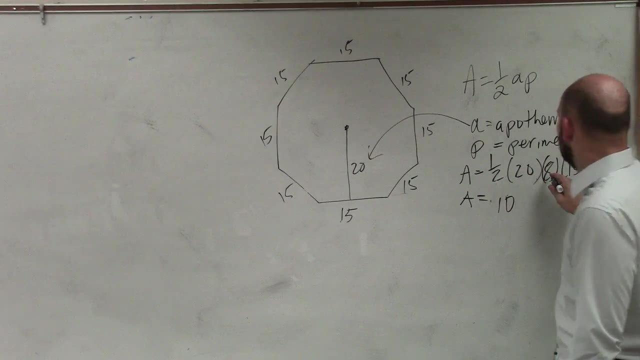 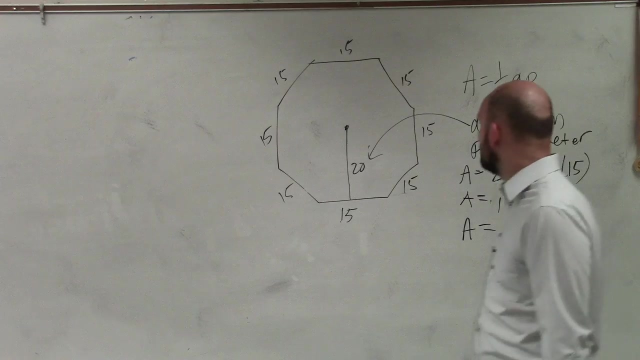 half is 60.. So I have a equals. let's do it this way: One half times 20 is going to be 10.. 8 times 16 is 120.. And therefore, double up the zeros, A equals 1,200.. Oh, I didn't give any units, but that'll be OK. Oh, there's no units in it. 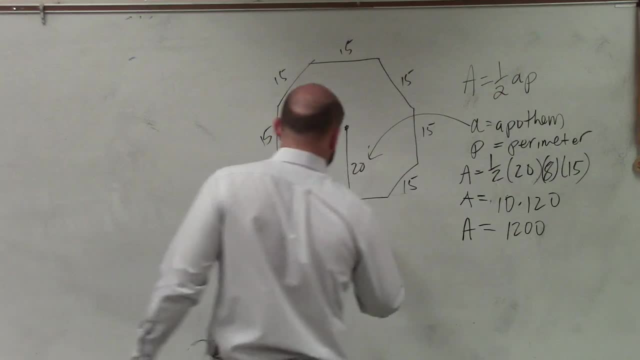 Well, there was units- Inches. So since we're still doing inches, it'll be inches squared. OK, You guys have four of those types of problems. I want you guys to do all those four types of problems. You guys have four of those types of problems, So I'm going to do all those four types.